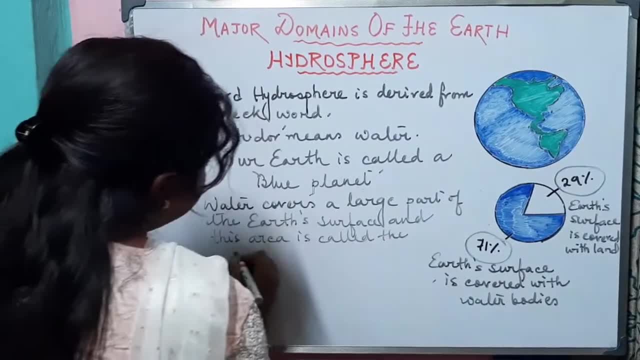 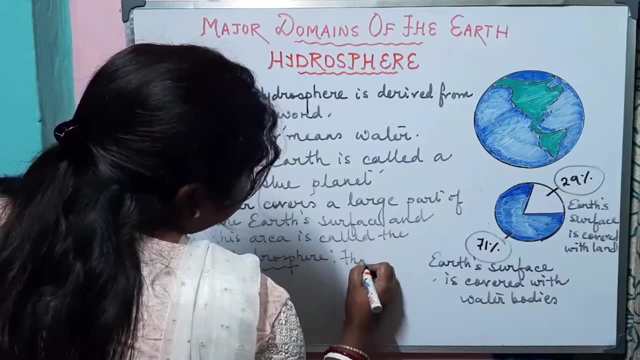 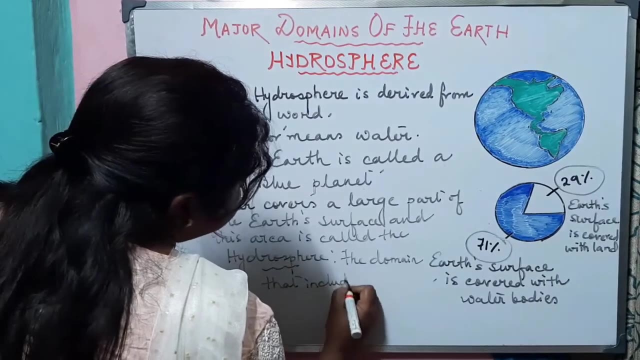 Don't worry, The name is accepted. We already have真els and enufere can never be any other. We know that they are animals: hydrosphere. so what is hydrosphere? hydrosphere is the domain that includes. 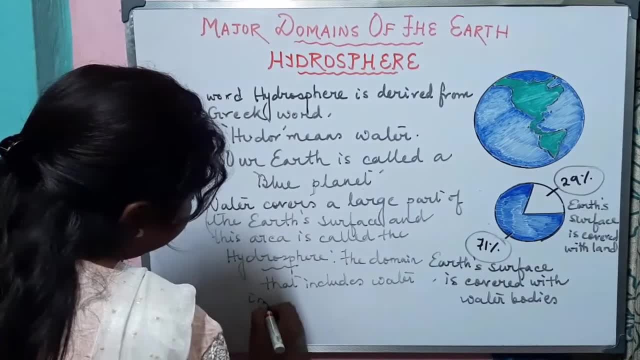 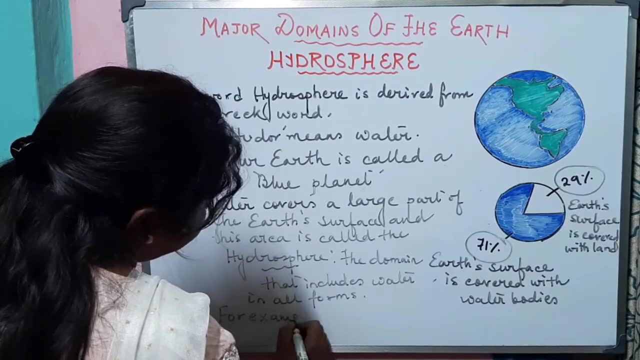 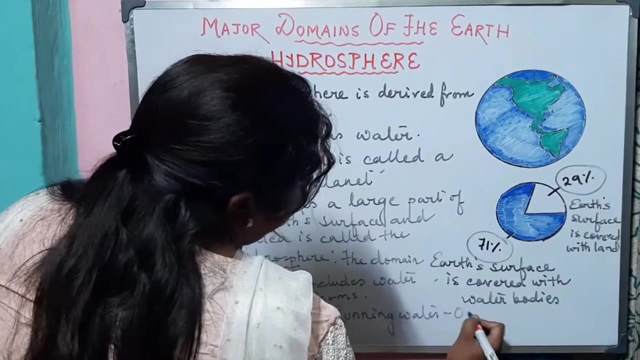 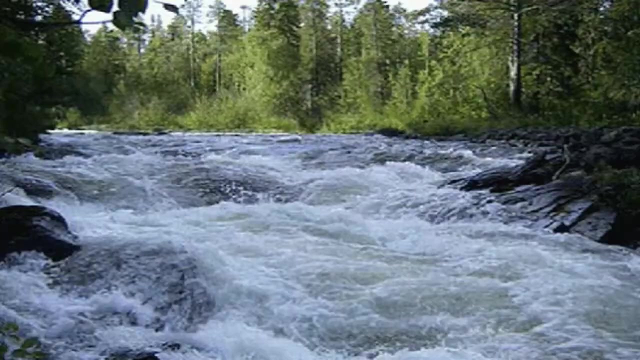 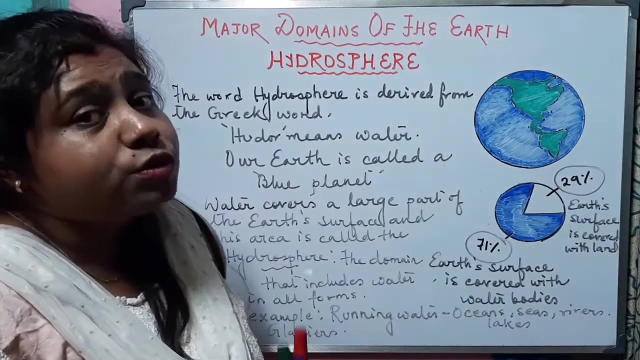 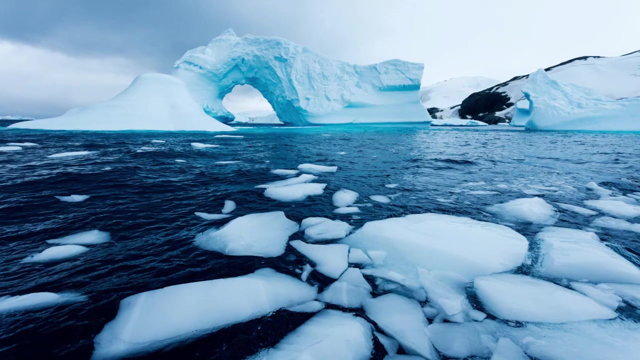 water in all forms, for example running water. where do we find the running water? in oceans, seas, rivers, lakes, in glaciers. now, what are glaciers? glaciers are huge masses of ice and water- ice when the water in its liquid form cools down and when the temperature comes down to around zero degrees Celsius. the 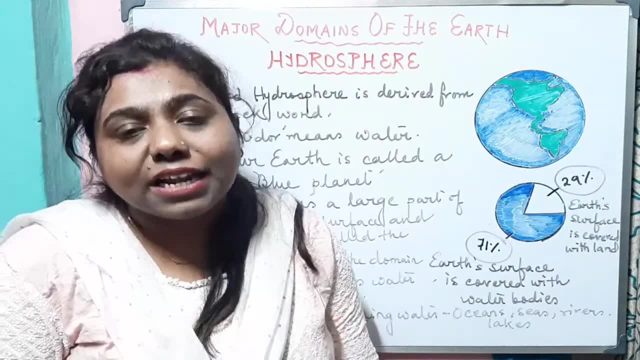 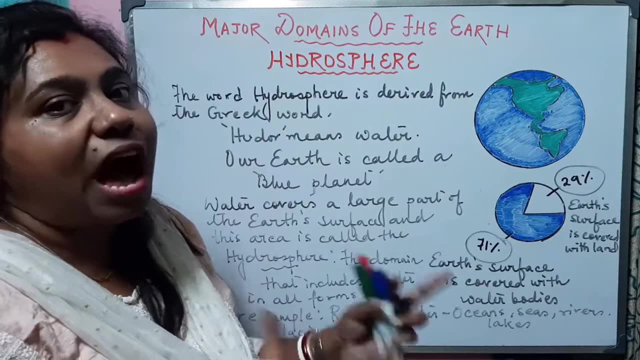 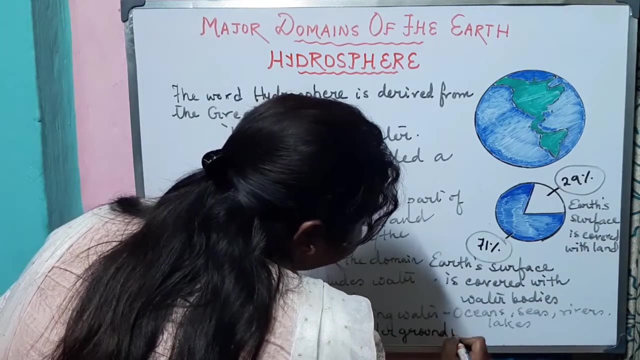 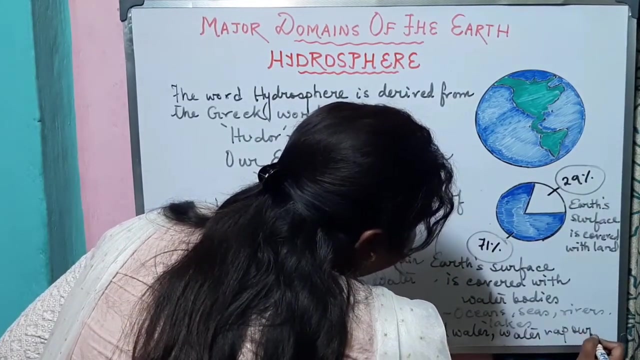 molecules stick together to form solid and that solid is ice. so we can understand that is a form from water and huge masses of ice forms glaciers. it also includes the underground waters and the water vapor in the atmosphere, so we can see that hydrosphere is the 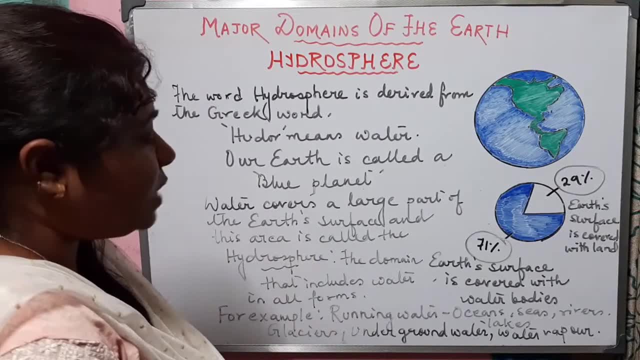 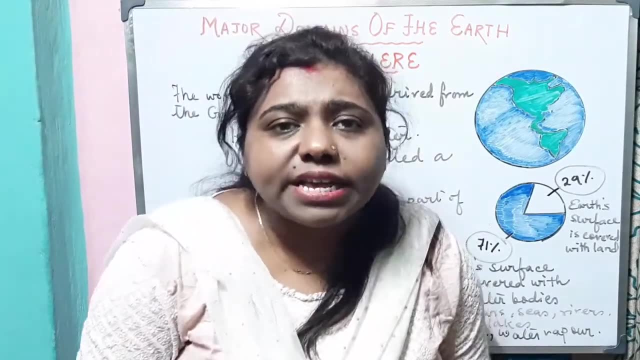 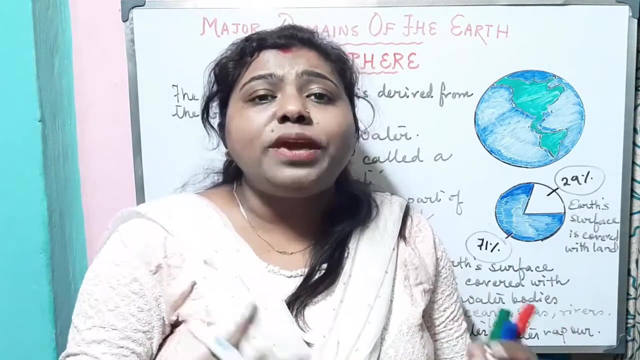 domain. that includes water in all forms. for example, the liquid form is ice, so we have form that is running water, glaciers, underground water, water vapor, everything. now the question that arises in your mind is that if we have so much water available, then why do we face the 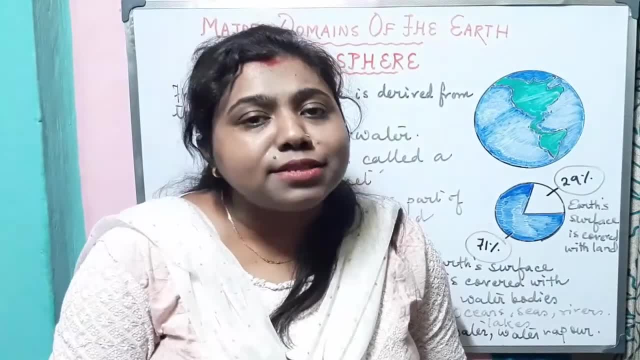 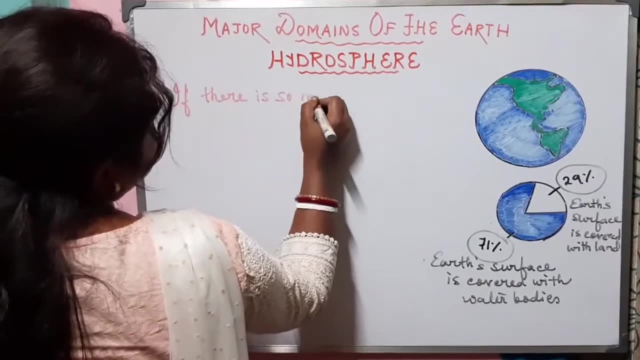 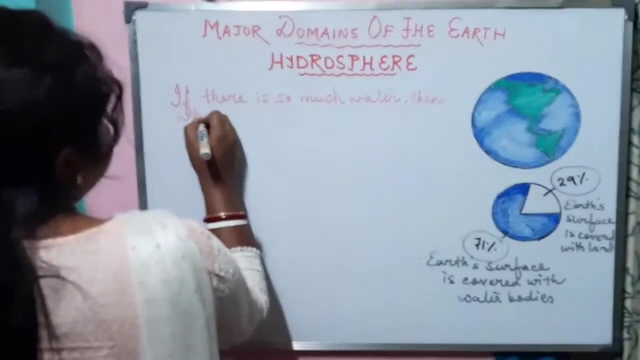 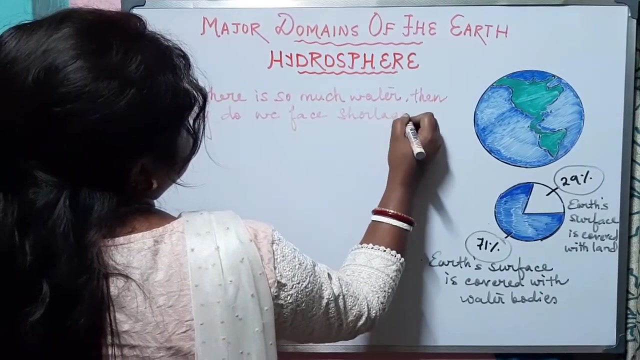 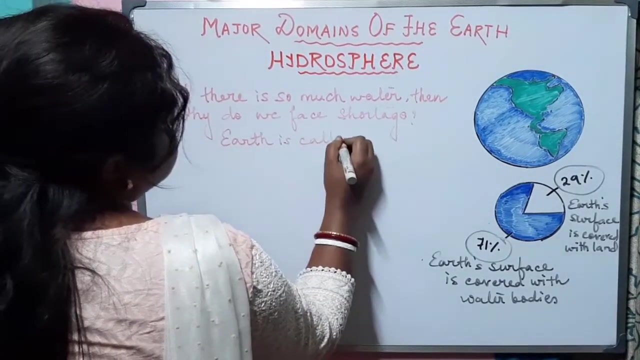 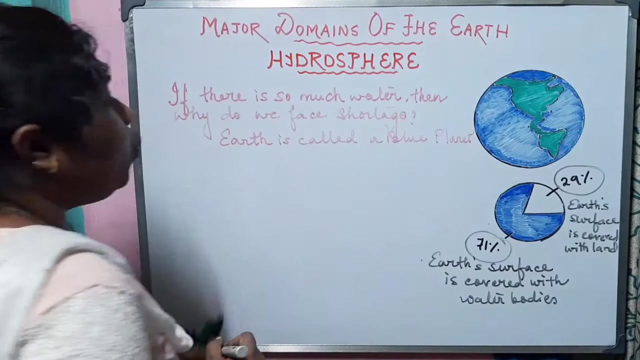 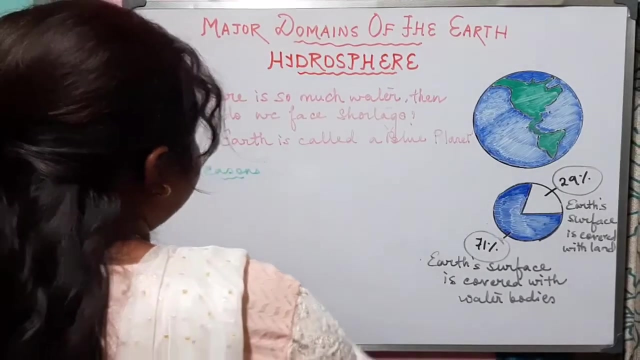 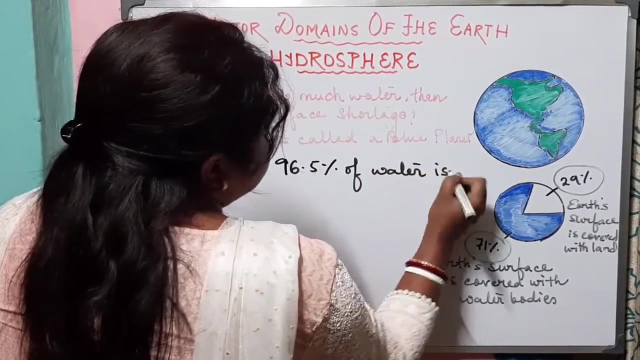 shortage of water? now let us find out the answer of this question. if there is so much water, then why do we face shortage, as we all know that earth is called a blue planet, but still we face shortage. now let us find out the reasons now. ninety six point five percent of water is found in oceans, and 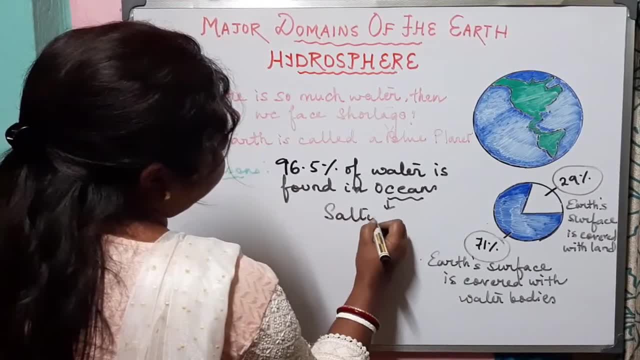 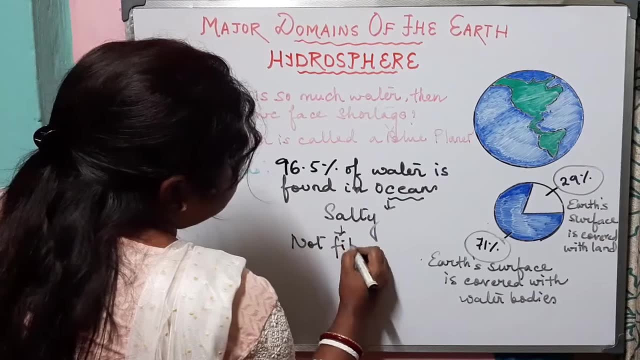 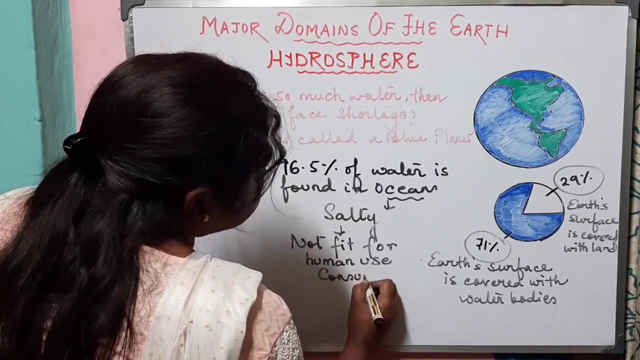 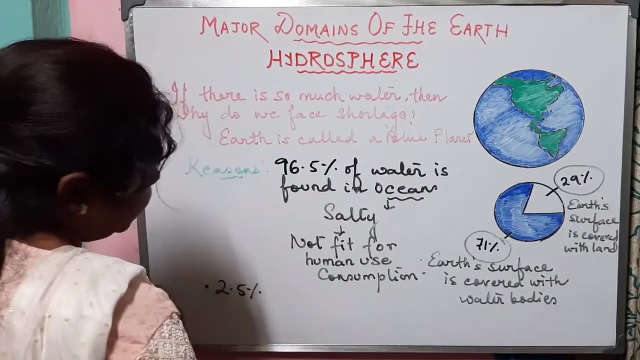 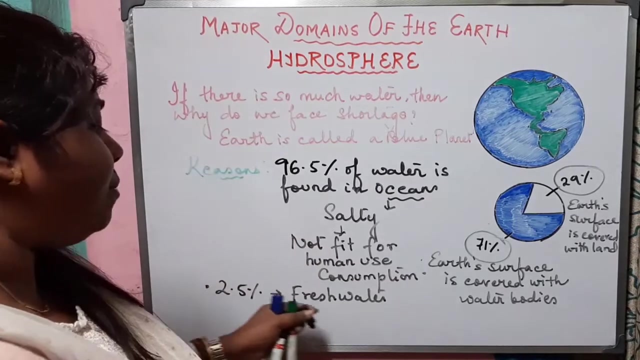 this water is salty. now can we drink this water? no, so this is not fit for water human use, that is, for our consumption. now remaining two point five percent is the fresh water. so you can see that only two point five percent is the fresh water. now seventy percent. 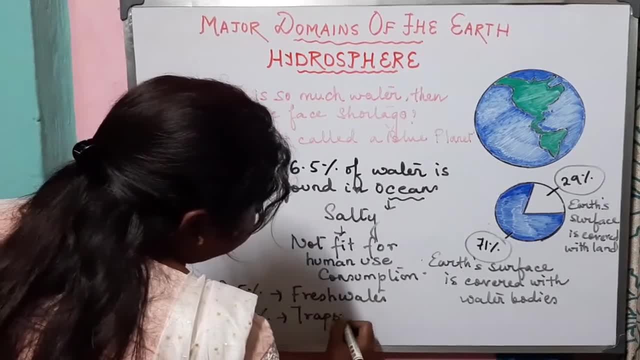 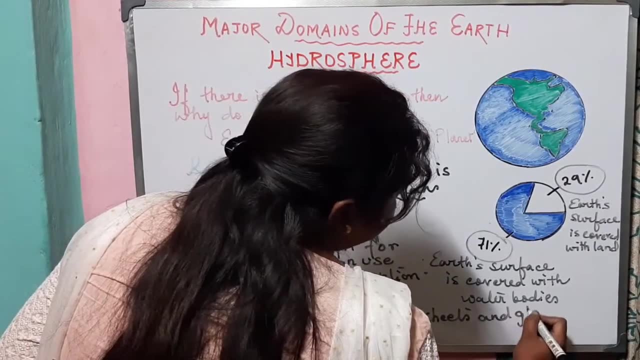 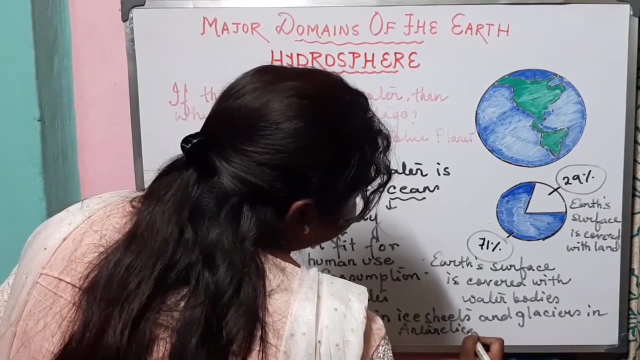 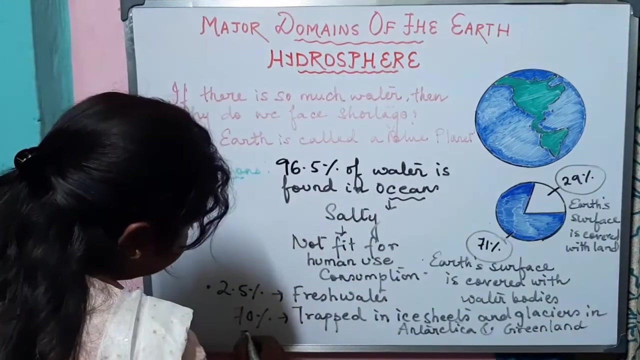 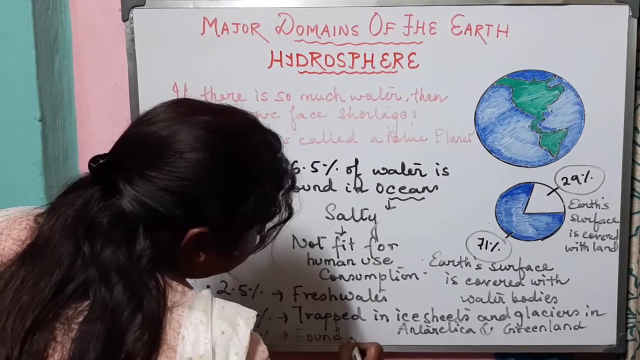 of the fresh water is trapped in ice. of the fresh water is trapped in ice sheets and glaciers in Antarctica and Greenland, and little less than thirty percent is found as underground water. so this is the reason why we face shortage now. ninety six point five percent of water is found in oceans and 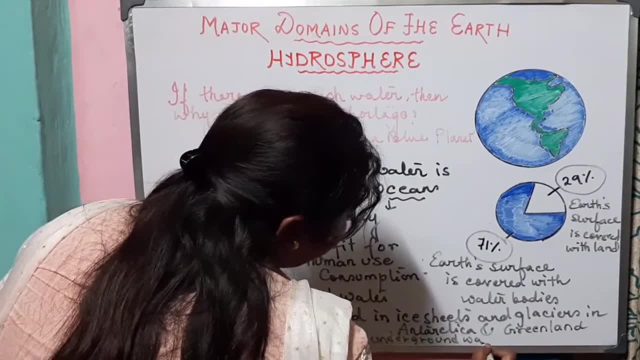 this water is salty now. ninety six point five percent is the fresh water now. seventy point five percent is the fresh water now. seventy six point five percent is the fresh water now. ninety six point five percent is the fresh water now. ninety six point five percent is the fresh water now. ninety six point five percent is the fresh water now. 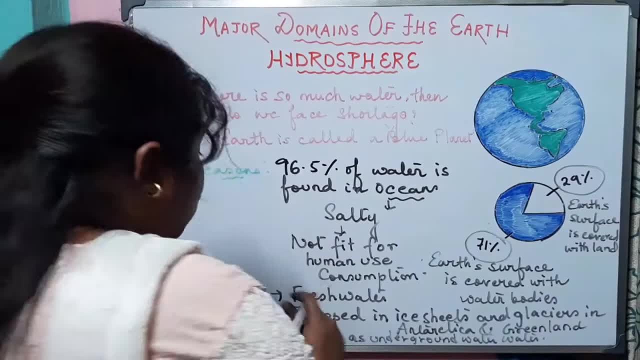 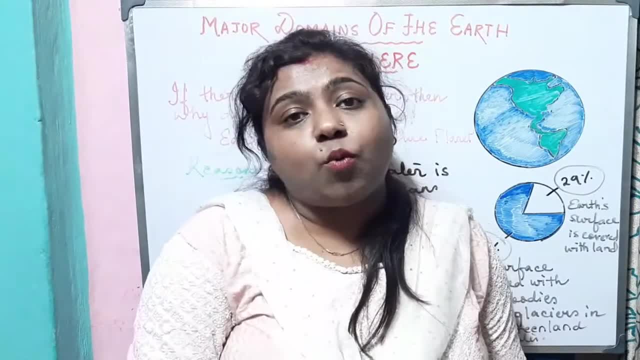 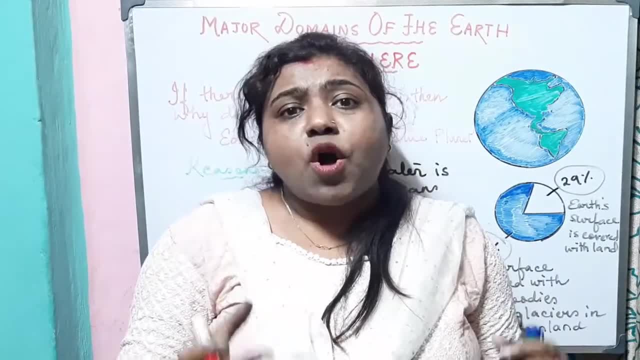 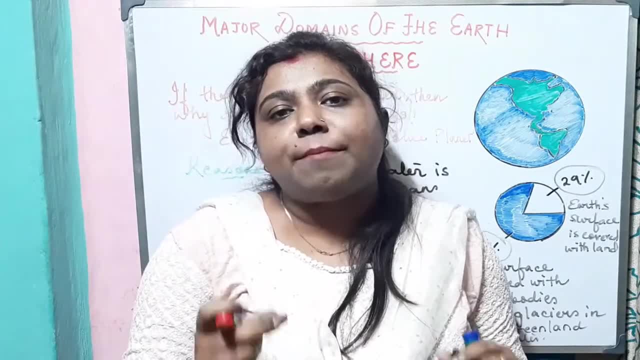 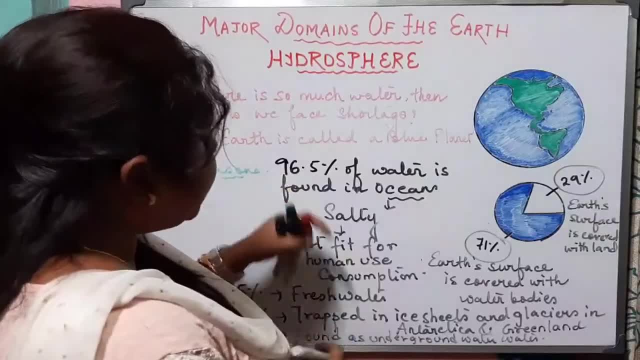 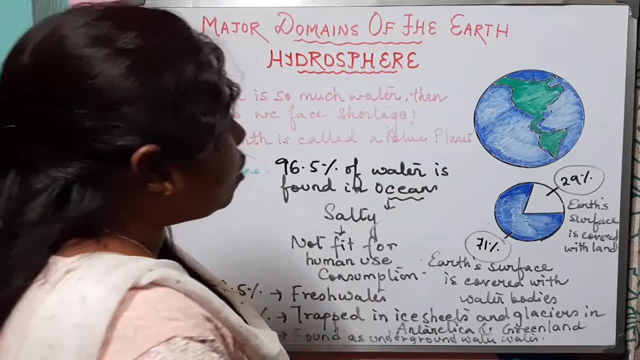 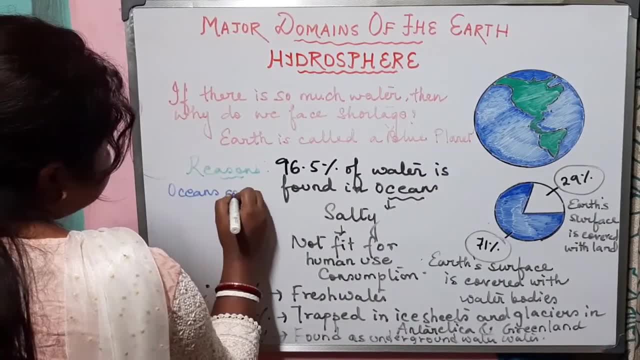 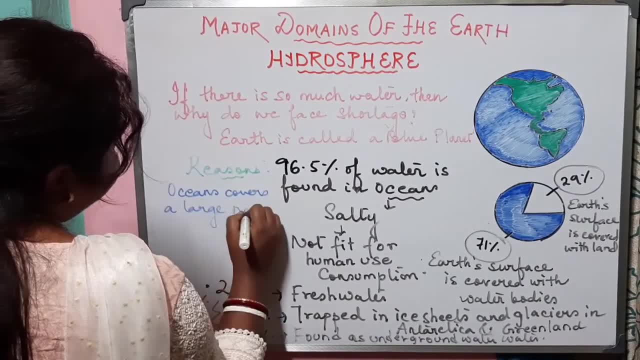 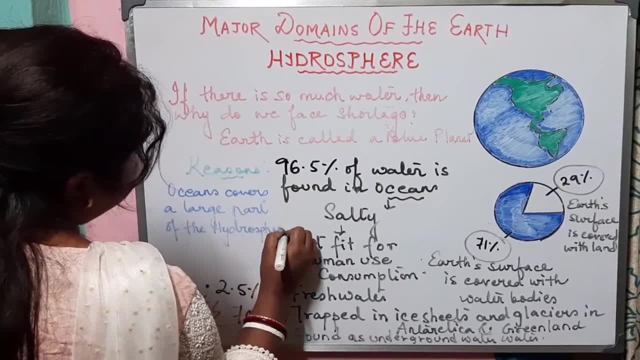 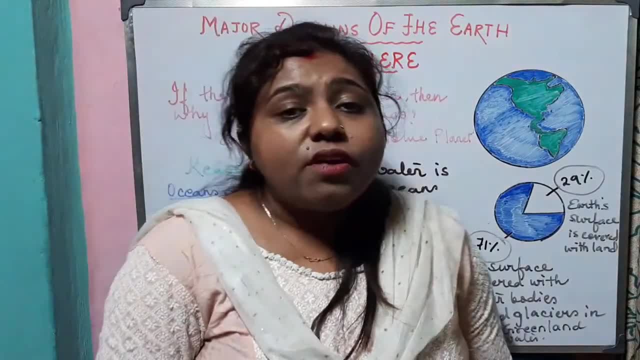 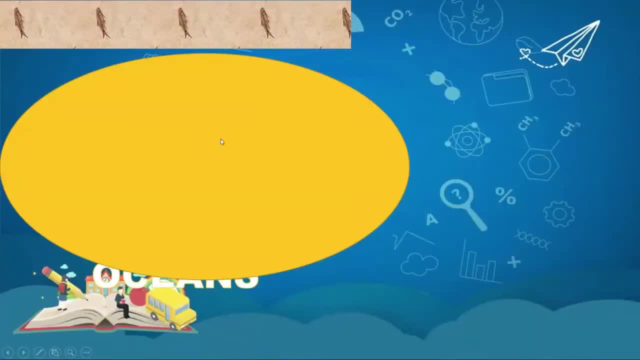 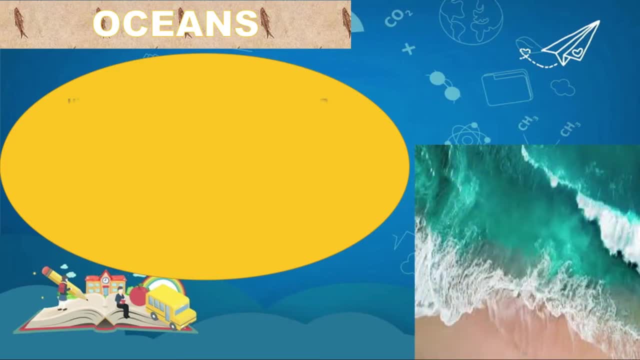 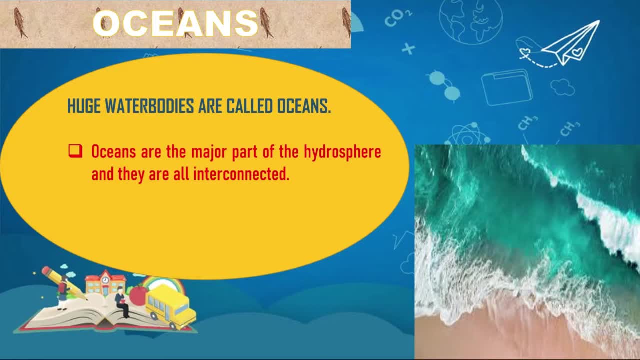 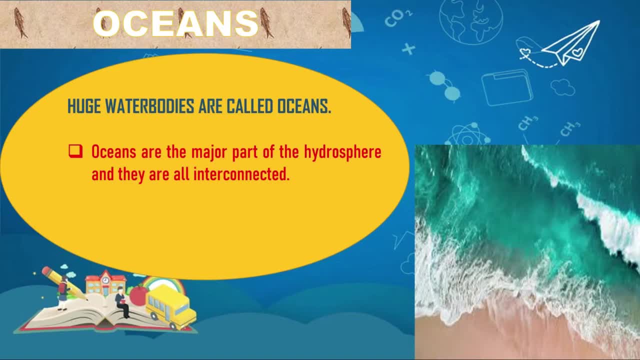 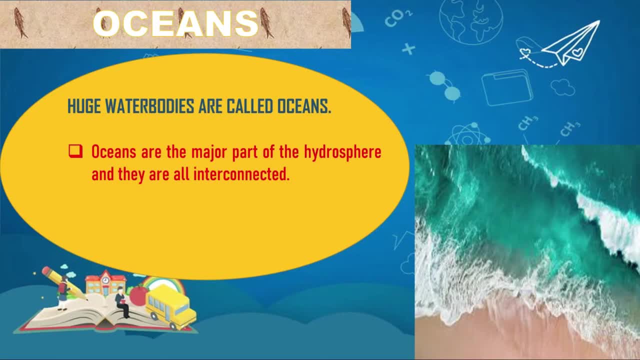 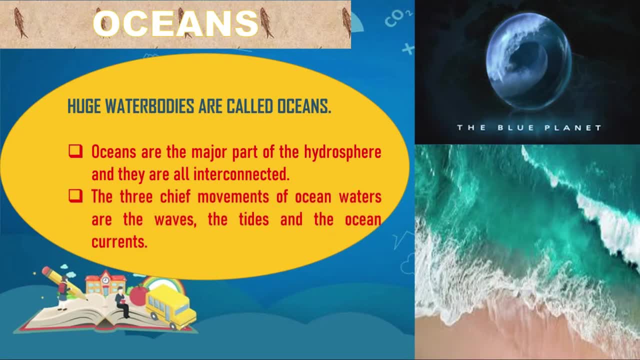 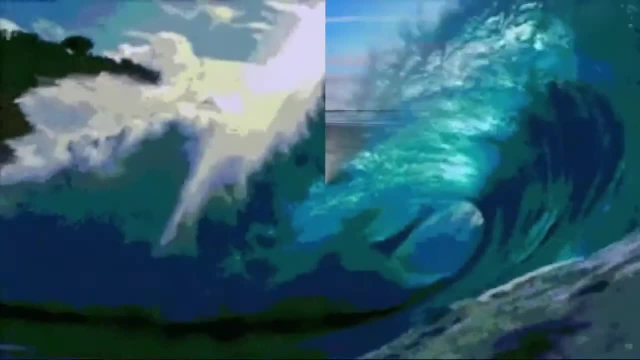 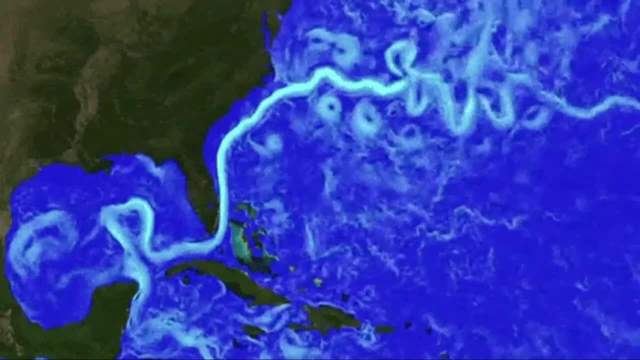 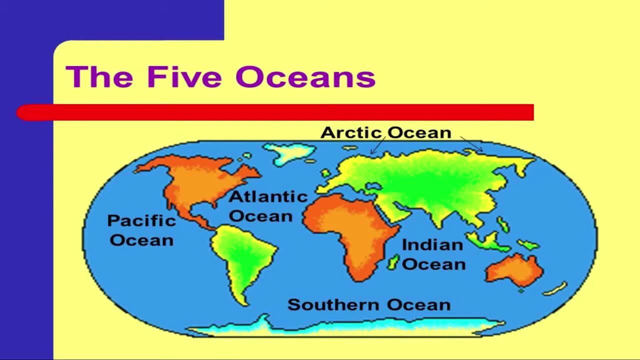 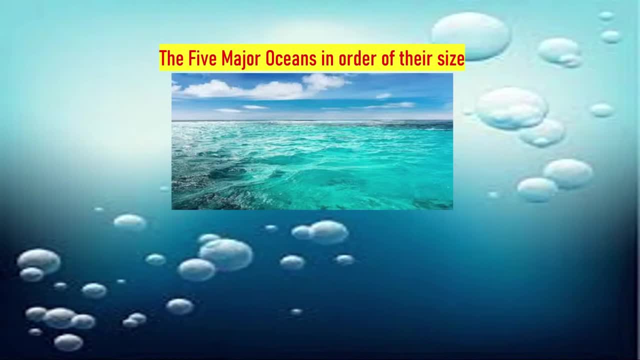 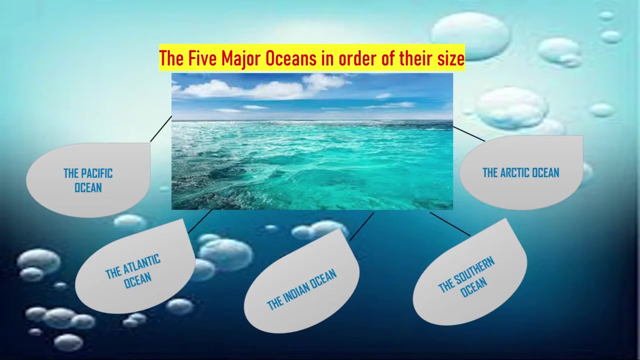 in the world. the five major oceans in the world, in order of their size, are: number one, the Pacific Ocean, which is the largest ocean in the world. number two, the Atlantic Ocean. number three, the Indian Ocean. number four, the Southern Ocean and number five, the Arctic Ocean, which is the smallest ocean in the world. 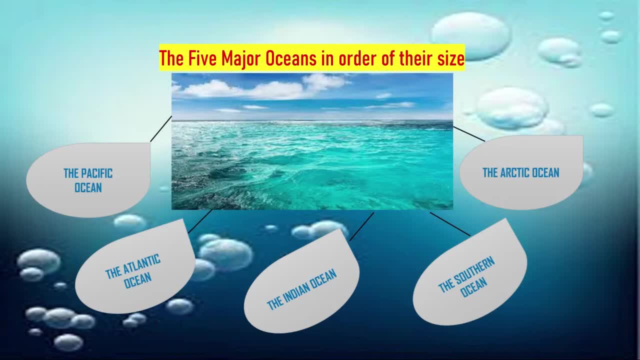 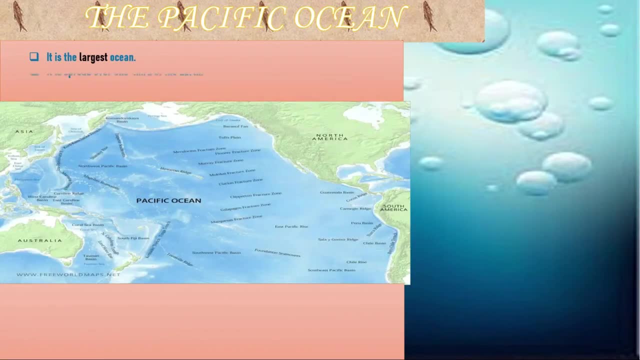 now let us know about each of this ocean one by one. the Pacific Ocean. the Pacific Ocean is the largest ocean in the world. it is spread over one-third of the earth and the depth of the Pacific Ocean is 10,994 meter. interestingly, the shape of the Pacific Ocean is almost circular. now let us know which are the 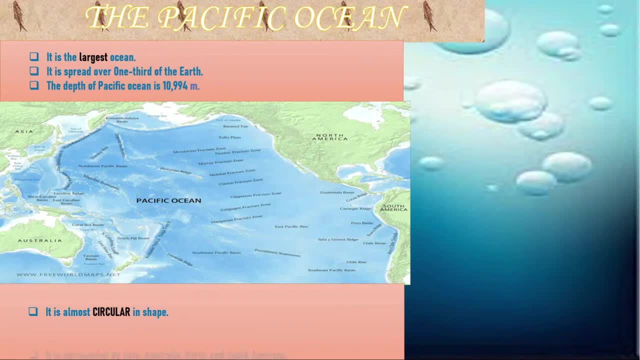 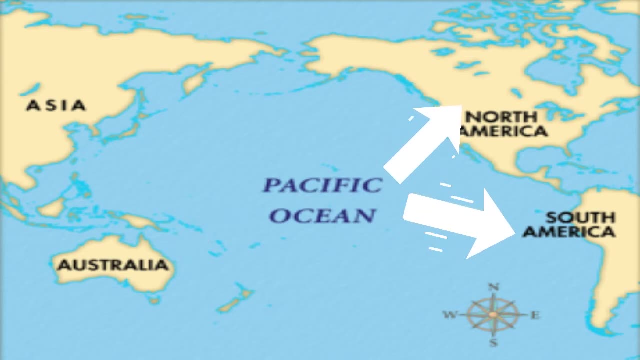 continents that surrounds the Pacific Ocean. the Pacific Ocean is surrounded by the Pacific Ocean and the Pacific Ocean is surrounded by the Pacific Ocean. and the Pacific Ocean is surrounded by the continent of Asia, Australia North and continent of Asia, Australia North and continent of Asia, Australia North and South America. now it's time to know an. 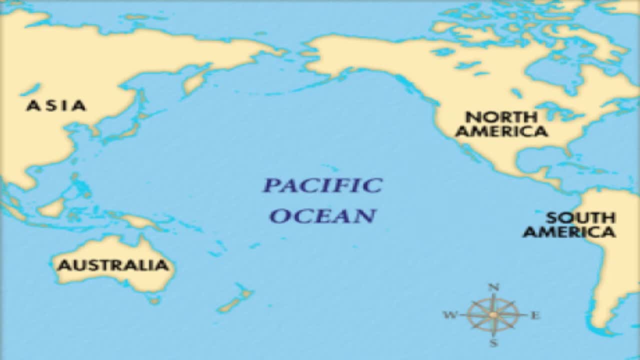 South America. now it's time to know an South America. now it's time to know an interesting and important fact about the interesting and important fact about the interesting and important fact about the Pacific Ocean. the deepest part of the Pacific Ocean, the deepest part of the Pacific Ocean, the deepest part of the earth, the Mariana Trench, with a depth of 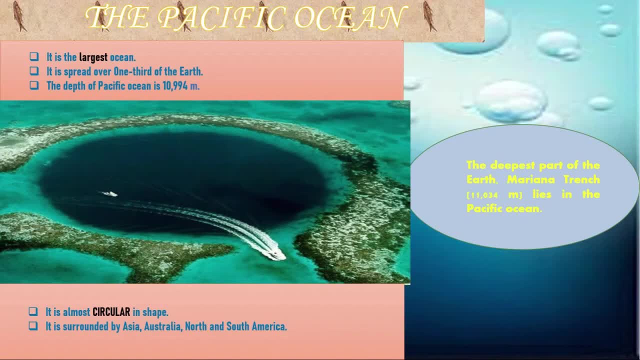 earth. the Mariana Trench, with a depth of earth. the Mariana Trench, with a depth of 11,000 34 meter, lies in the Pacific. 11,000 34 meter lies in the Pacific. 11,000 34 meter lies in the Pacific Ocean. now let us move ahead with our next. 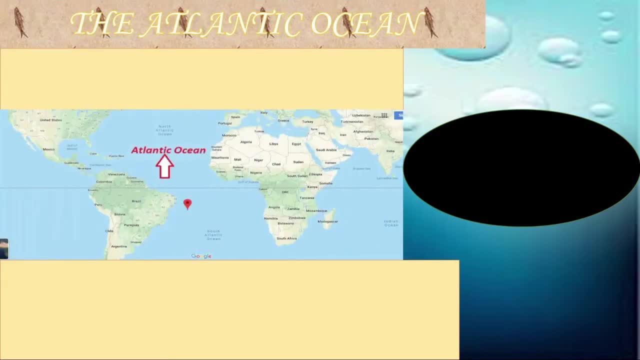 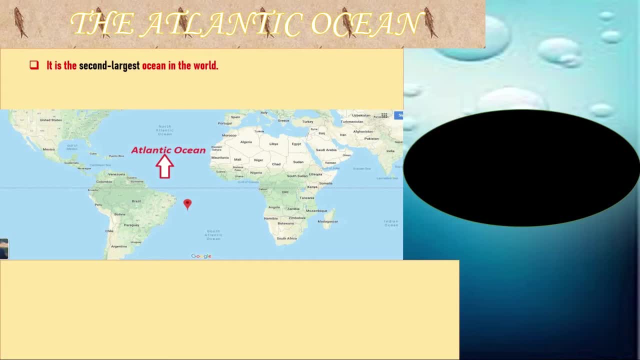 interestingly, if you will have a look. interestingly, if you will have a look on the map, you will see that the shape of on the map, you will see that the shape of on the map, you will see that the shape of the Atlantic Ocean is exactly like the. 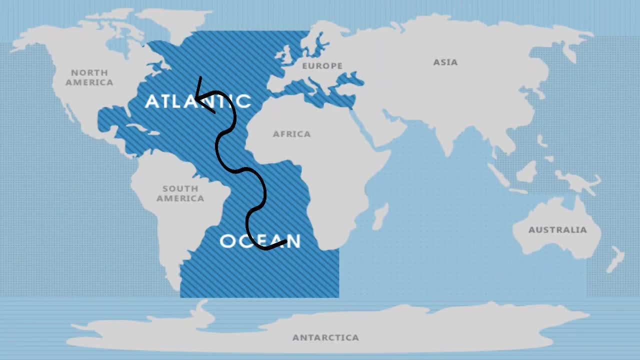 the Atlantic Ocean is exactly like the. the Atlantic Ocean is exactly like the alphabet s, so we can say that the alphabet s. so we can say that the alphabet s. so we can say that: the Atlantic Ocean is s-shaped, now, let us. Atlantic Ocean is s-shaped now, let us. 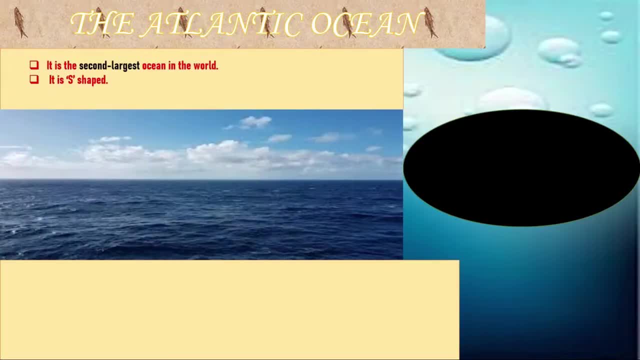 Atlantic Ocean is s-shaped. now, let us know about the depth of the Atlantic. know about the depth of the Atlantic, know about the depth of the Atlantic Ocean. the depth of the Atlantic Ocean is Ocean. the depth of the Atlantic Ocean is Ocean. the depth of the Atlantic Ocean is the busiest ocean, and let us know why. 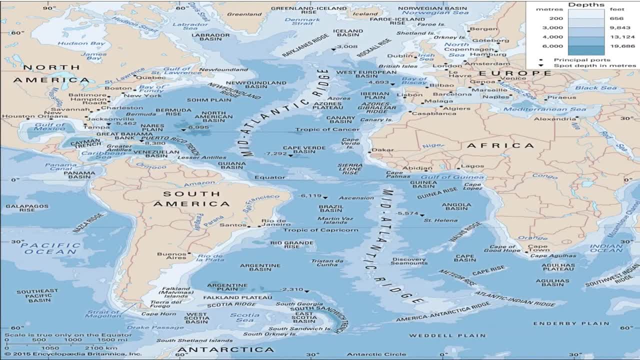 the busiest ocean. and let us know why the busiest ocean? and let us know why now. what does it mean? it means that the now. what does it mean? it means that the now. what does it mean? it means that the place where the Atlantic Ocean meets, place where the Atlantic Ocean meets. 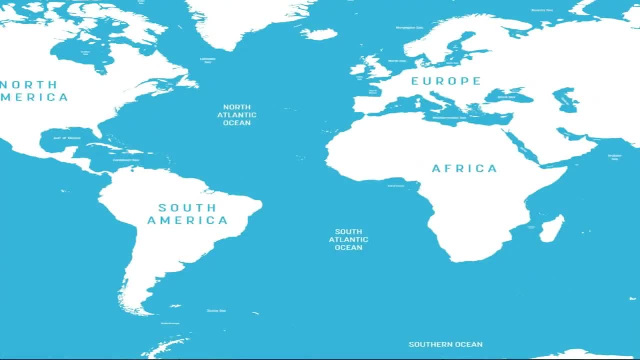 place where the Atlantic Ocean meets with the land. it is intended. that means with the land. it is intended. that means with the land. it is intended. that means it has ridges. this is called coastline. it has ridges. this is called coastline. it has ridges. this is called coastline. that means the zone where the land meets. 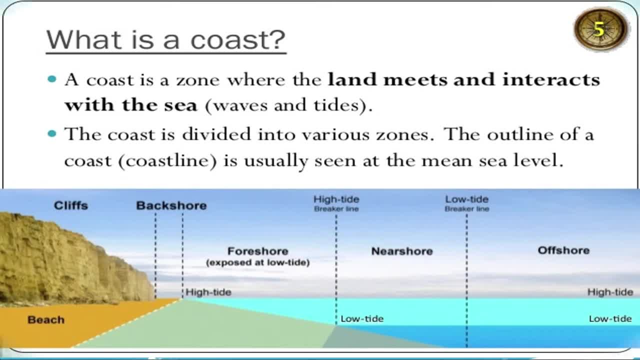 that means the zone where the land meets, that means the zone where the land meets and interacts with the sea. so we can say and interacts with the sea. so we can say and interacts with the sea. so we can say that the coastline of the Atlantic Ocean, that the coastline of the Atlantic Ocean is not smooth but it is intended. the 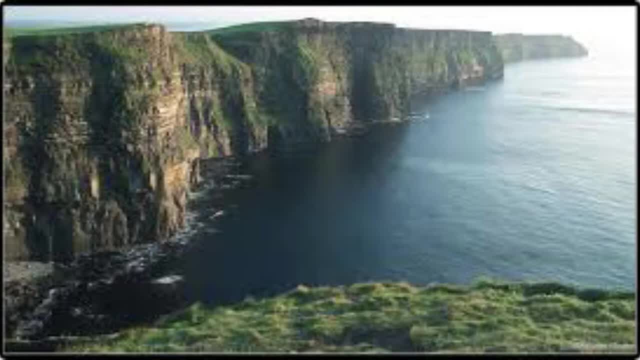 is not smooth but it is intended. the is not smooth but it is intended. the coastline of the Atlantic Ocean is highly coastline of the Atlantic Ocean is highly coastline of the Atlantic Ocean is highly intended. so this irregular and intended intended so this irregular and intended intended so this irregular and intended coastline provides ideal location for 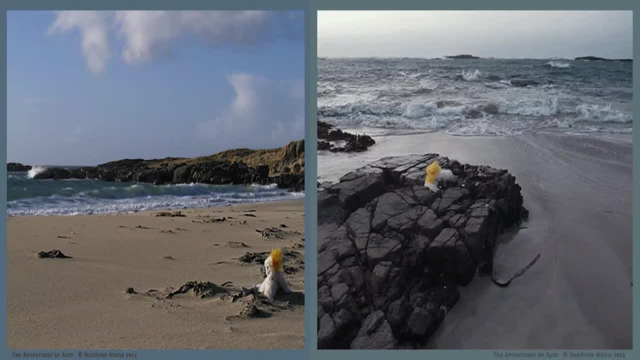 coastline provides ideal location for coastline, provides ideal location for natural ports and harbors, and this makes natural ports and harbors and this makes natural ports and harbors and this makes Atlantic Ocean the busiest ocean from Atlantic Ocean, the busiest ocean from Atlantic Ocean, the busiest ocean from the point of view of commerce. now let us 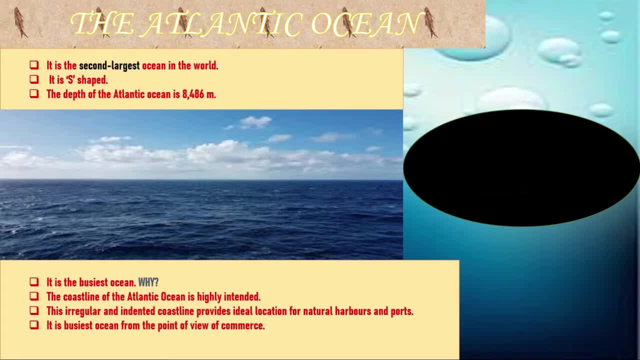 the point of view of commerce. now, let us the point of view of commerce. now, let us know which are the continents that know, which are the continents that know, which are the continents that surrounds Atlantic Ocean. Atlantic Ocean surrounds Atlantic Ocean. Atlantic Ocean surrounds Atlantic Ocean. Atlantic Ocean is flanked by the North and the South. 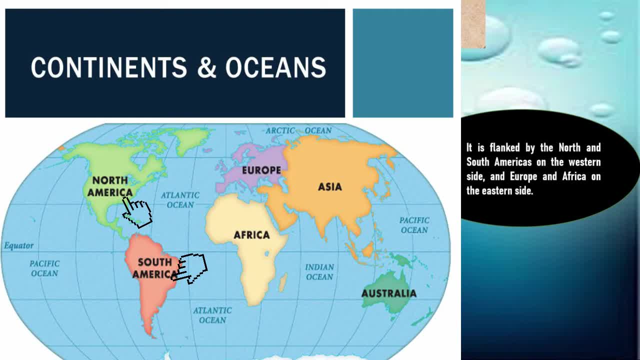 is flanked by the North and the South is flanked by the North and the South, Americas on the western side and Europe, Americas on the western side, and Europe, Americas on the western side. and Europe and Africa on the eastern side, now let. and Africa on the eastern side, now let. 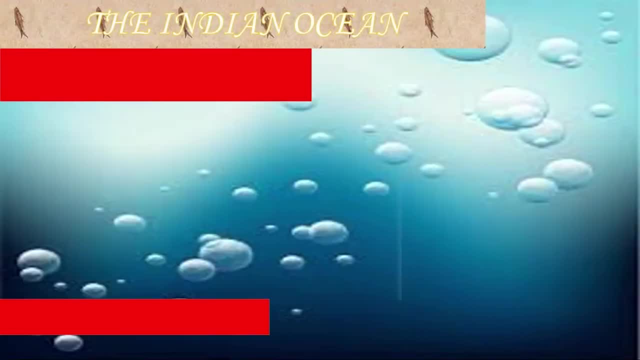 and Africa on the eastern side. now let us move ahead with the next ocean. the us move ahead with the next ocean. the us move ahead with the next ocean: the Indian Ocean. the Indian Ocean is a third Indian Ocean. the Indian Ocean is a third Indian Ocean. the Indian Ocean is a third largest ocean and it is the only ocean. 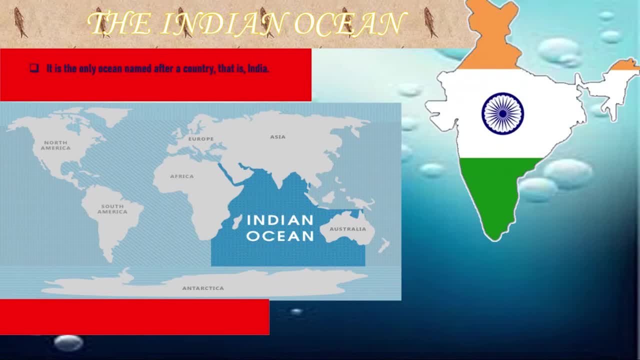 largest ocean and it is the only ocean, largest ocean, and it is the only ocean which is named after a country, that is, which is named after a country that is, which is named after a country that is India, and we all should be proud of that India, and we all should be proud of that. 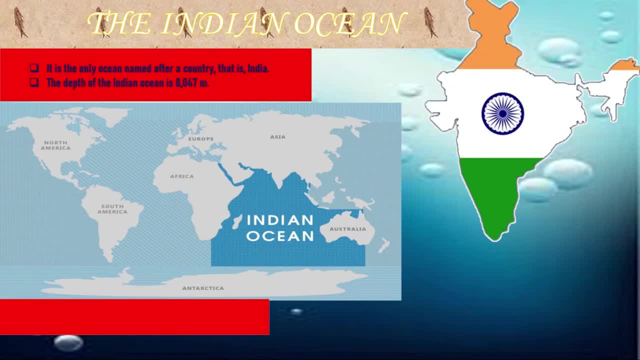 India and we all should be proud of that. the Indian Ocean has a depth of 8047. the Indian Ocean has a depth of 8047. the Indian Ocean has a depth of 8047 meter. the shape of the Indian Ocean is meter. the shape of the Indian Ocean is: 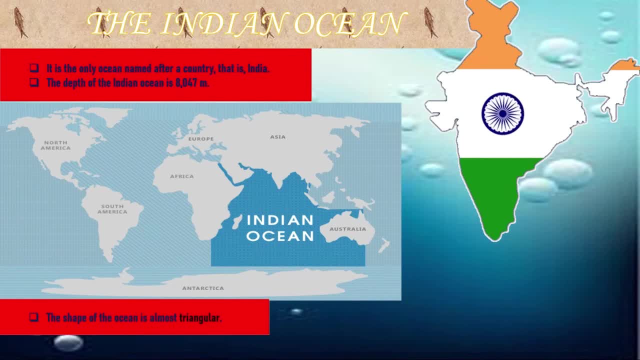 meter. the shape of the Indian Ocean is almost triangular now. let us know which almost triangular now. let us know which almost triangular now. let us know which are the continents that surrounds Indian. are the continents that surrounds Indian? are the continents that surrounds Indian Ocean? the Indian Ocean is surrounded by 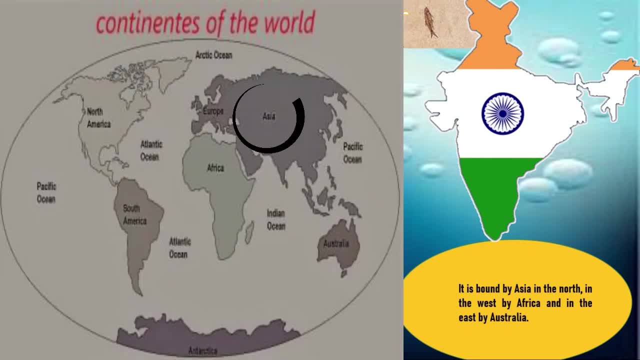 Ocean. the Indian Ocean is surrounded by Ocean. the Indian Ocean is surrounded by the continent of Asia in the north, in the continent of Asia in the north, in the continent of Asia in the north, in the West, by Africa and in the East, by the West, by Africa and in the East by. 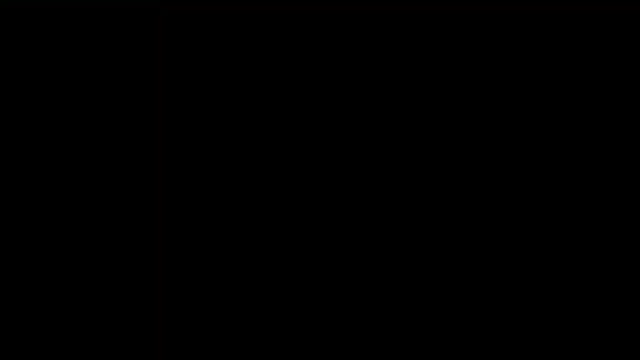 the West by Africa and in the East by Australia. now let us move ahead the Australia. now let us move ahead. the Australia, now let us move ahead. the next ocean, that is the southern ocean. next ocean, that is the southern ocean. next ocean, that is the southern ocean. the southern ocean is also known as the 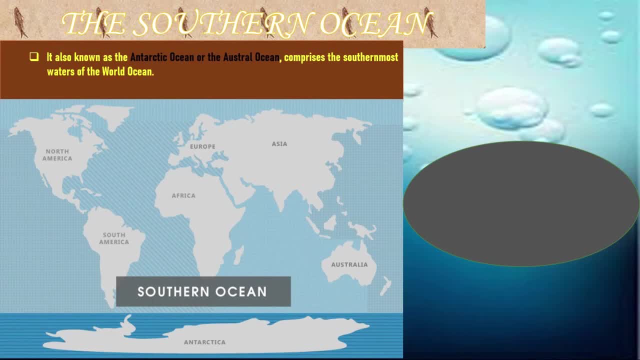 the southern ocean is also known as the. the southern ocean is also known as: the Antarctic Ocean on the Austral Ocean. Antarctic Ocean on the Austral Ocean. Antarctic Ocean on the Austral Ocean, which comprises the southernmost waters, which comprises the southernmost waters, which comprises the southernmost waters of the world oceans. the depth of. 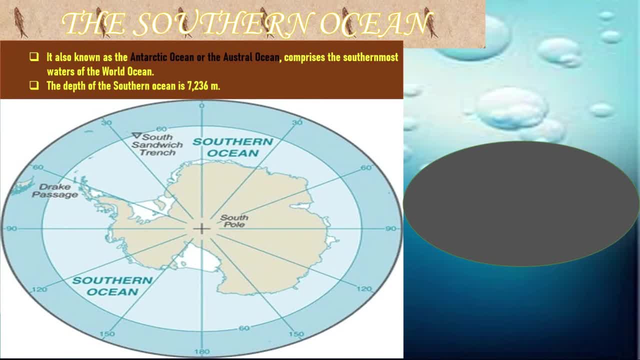 of the world oceans, the depth of of the world oceans, the depth of southern ocean is 7236 meter now. let us southern ocean is 7236 meter now. let us southern ocean is 7236 meter now. let us know that the southern ocean surrounds, know that the southern ocean surrounds. 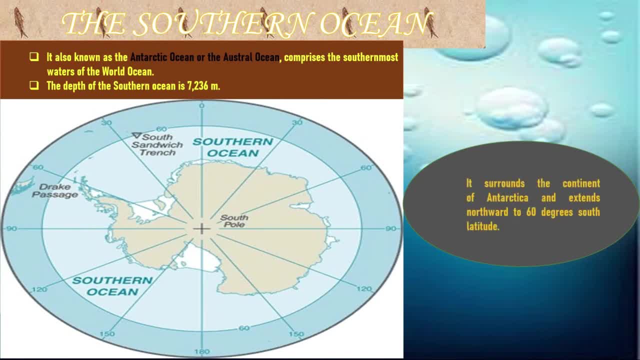 know that the southern ocean surrounds which continent? the southern ocean? which continent? the southern ocean? which continent? the southern ocean surrounds the continent of Antarctica and surrounds the continent of Antarctica. and surrounds the continent of Antarctica and extends northward to 60 degrees south. extends northward to 60 degrees south. 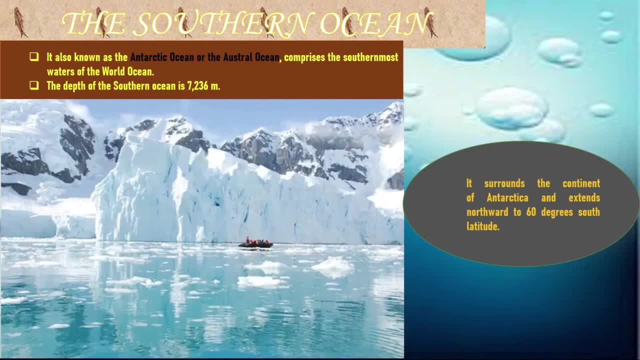 extends northward to 60 degrees south latitude now. let us move ahead with the latitude now. let us move ahead with the latitude now. let us move ahead with the next ocean: the Arctic Ocean. the Arctic next ocean: the Arctic Ocean. the Arctic next ocean: the Arctic Ocean. the Arctic Ocean is located within the Arctic Circle. 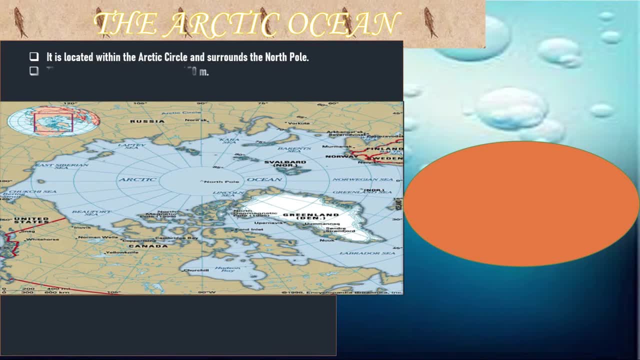 Ocean is located within the Arctic Circle. Ocean is located within the Arctic Circle and surrounds North Pole. the depth of, and surrounds North Pole, the depth of, and surrounds North Pole. the depth of the Arctic Ocean is 5,450 meter and it is. the Arctic Ocean is 5,450 meter and it is. 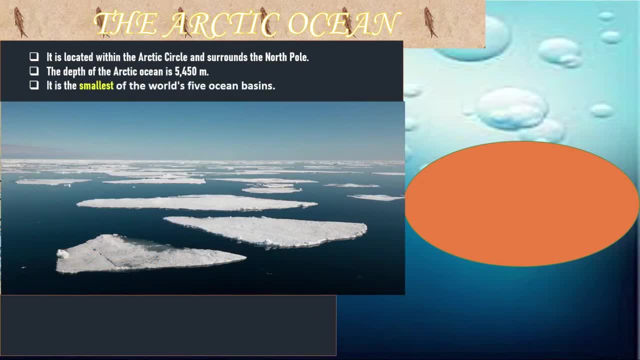 the Arctic Ocean is 5,450 meter and it is the smallest on the walls five ocean, the largest on the walls five ocean, the largest on the walls five ocean basins. it is bounded by northern coast of basins. it is bounded by northern coast of. 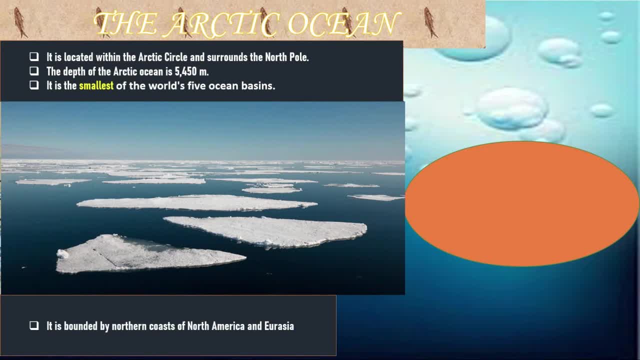 basins. it is bounded by northern coast of North America and Eurasia. now it's time, North America and Eurasia, now it's time, North America and Eurasia. now it's time to know an interesting and important to know an interesting and important to know an interesting and important fact about the Arctic Ocean, the Bering. 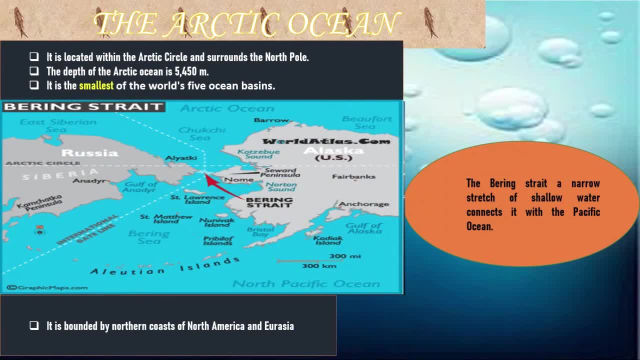 fact about the Arctic Ocean: the Bering fact about the Arctic Ocean. the Bering Strait and narrow stretch of shallow Strait and narrow stretch of shallow Strait and narrow stretch of shallow water connects the Arctic Ocean with the water. connects the Arctic Ocean with the water. connects the Arctic Ocean with the Pacific Ocean. we have already learned.